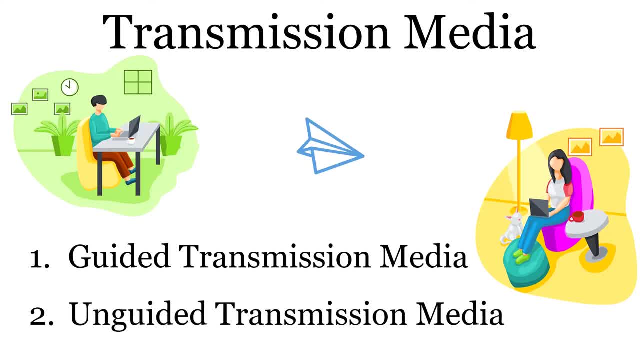 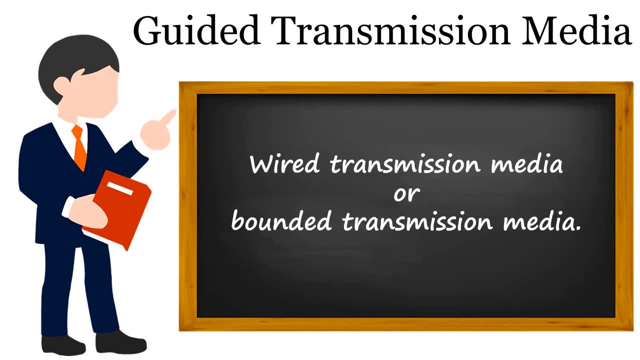 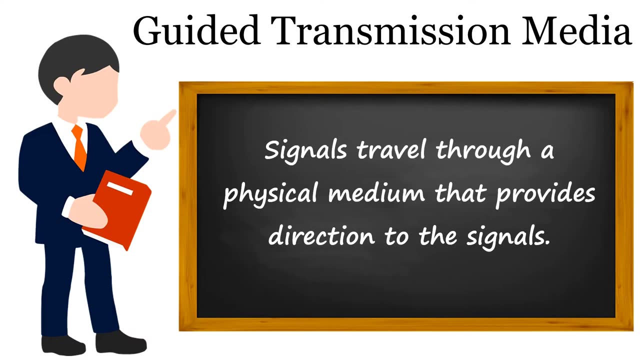 that is, guided transmission media and unguided transmission media. The guided transmission media is also referred as wired transmission media or bounded transmission media. Guided media provides a physical medium for signals to travel from source towards destination. As it uses physical conductor for signals to travel, it provides a particular direction to these signals. 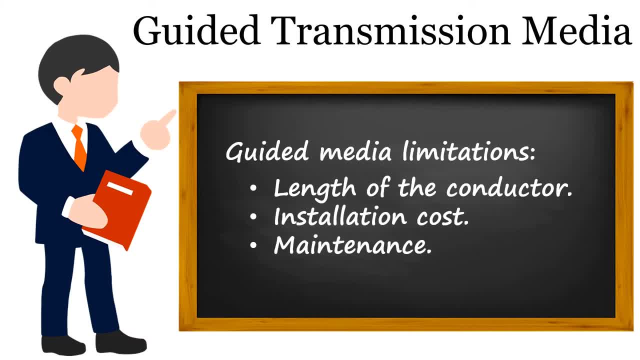 But, as we all know, the physical conductor have certain limitations, such as length of the conductor. Each conductor is produced up to a certain length And, as we all know, the physical conductor has certain limitations, such as length of the conductor, And it is not certain that a single length conductor would connect sender and receiver at once. 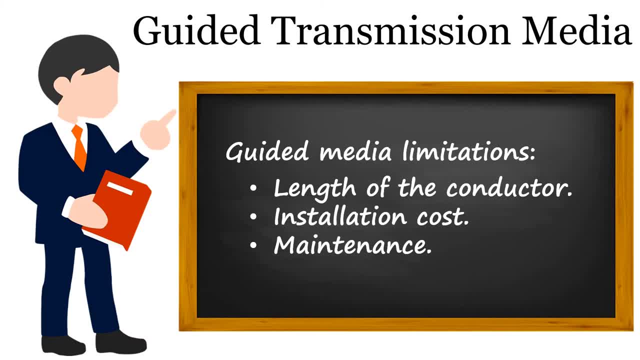 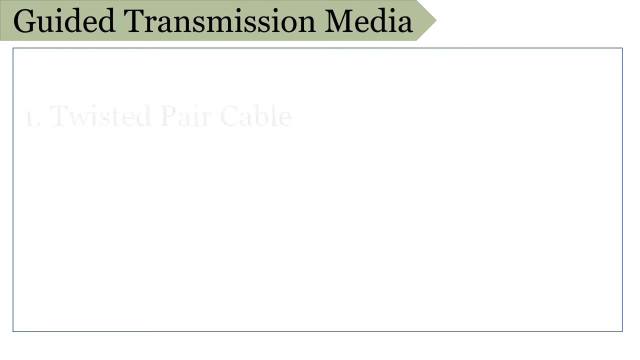 We may require a pitter to cover the area between sender and receiver. Other limitation is installation cost And of course the maintenance is also an issue with the guided media. The guided transmission media can be further categorized into three subcategories. The first one is twisted pair cable, that is, two insulated copper wire twisted around each other. 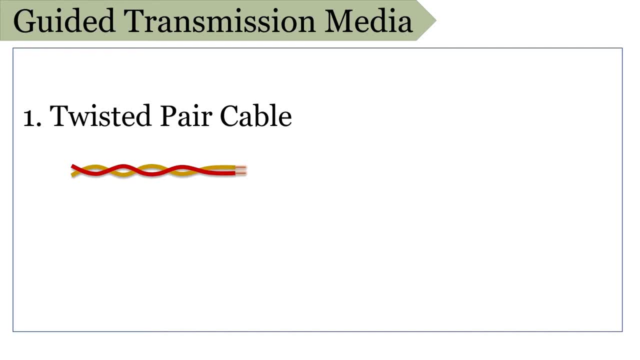 Comparatively to the other guided media, the twisted pair cable has low bandwidth and provide less protection from interference. The next one is coaxial cable. Here, an insulated copper wire is further encased with a metallic braid which act as a second conductor, completing the circuit. 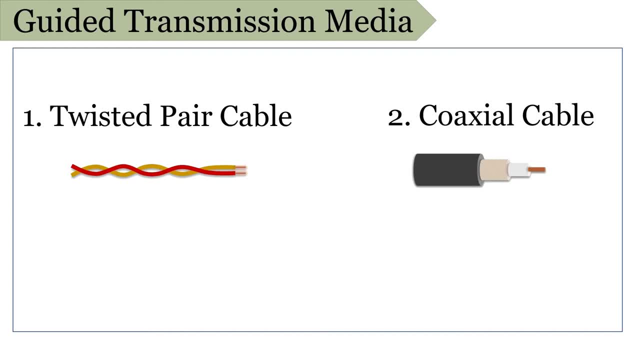 And also it provide protection against noise. This structure is further encased with an insulating material. The coaxial cable carries signal of higher frequency. The third subcategory is optical fiber. This fiber is made up of glass or plastic, And the signal here is transmitted in the form of light. 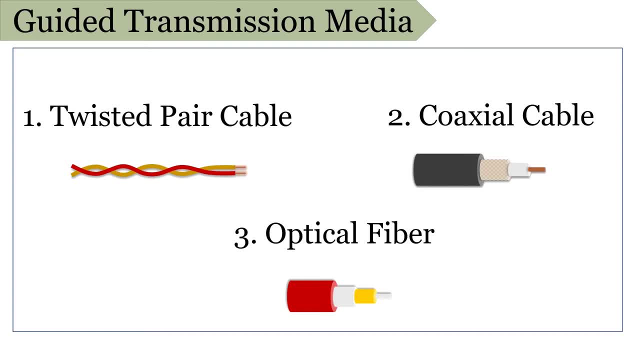 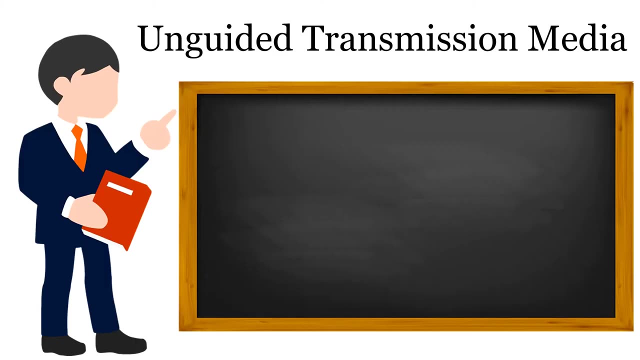 The optical fiber is noise resistance, has less signal attenuation and has a higher bandwidth Comparatively. it is expensive and require a installation and maintenance charge, And of course it is made up of glass. that's why it is also fragile. The other kind of transmission media is unguided transmission media. 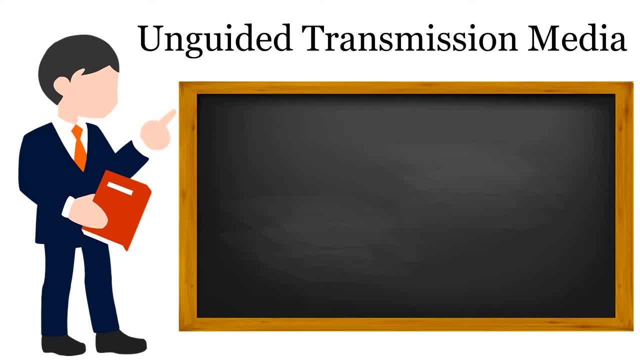 It is not possible to cover every geographical area Using guided transmission media Because of geographical conditions such as mountain, river, oceans, etc. The unguided transmission media provide a way of communication in such areas. It is also referred as wireless transmission media or unbounded transmission media. 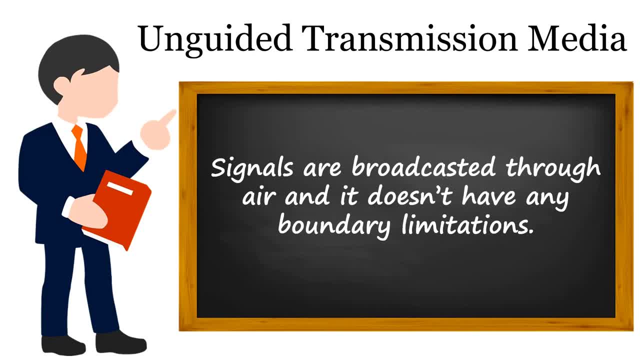 It doesn't require a physical medium, and signals are transmitted through air in the form of electromagnetic signals. The signals are broadcasted in the air And are captured by the devices Capable of receiving those signals. The signals does not have any boundary limitation. 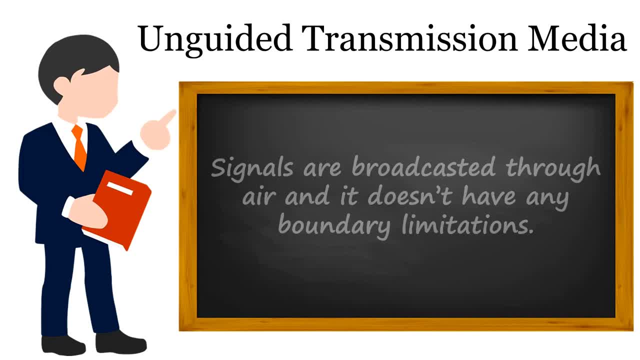 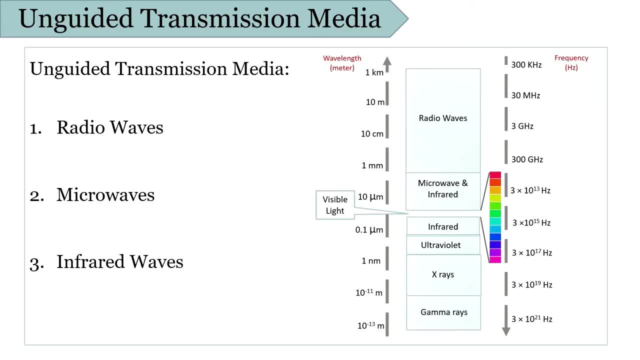 And are transmitted in every direction. User with a capable device can connect to the network from anywhere, anytime. The unguided transmission media is further categorized into three subcategories, That is, radio wave, microwave and infrared wave. Radio wave are low frequency signals and can travel a long distance. 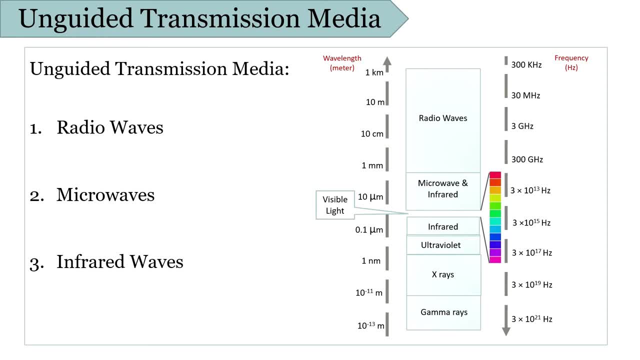 As it is a low frequency signal, It can easily penetrate the building or any obstacle easily. Thus it is usually used to send radio signals. The microwaves are transmitted in a straight line And hence it require line of sight transmission. The distance covered by microwave depend on the height of sender and receiver's antenna. 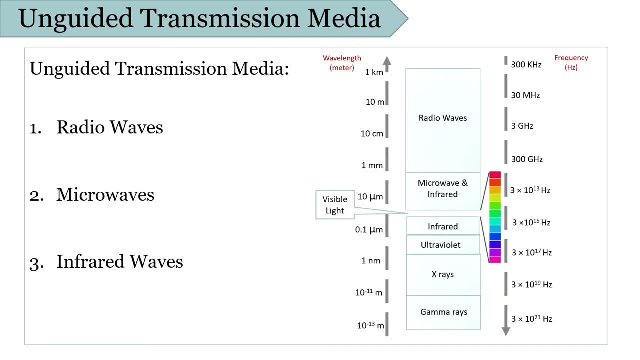 Taller is the height of antenna, longer is the distance covered. As these are high frequency wave, They are usually used by mobile phones, televisions etc. The infrared wave are even of higher frequency, Thus it cannot easily penetrate any obstacle, And are used by remote of televisions etc. 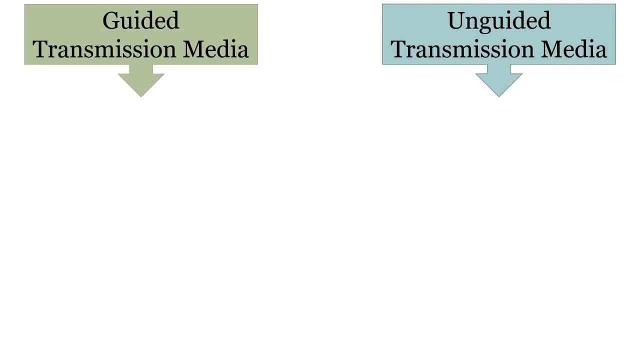 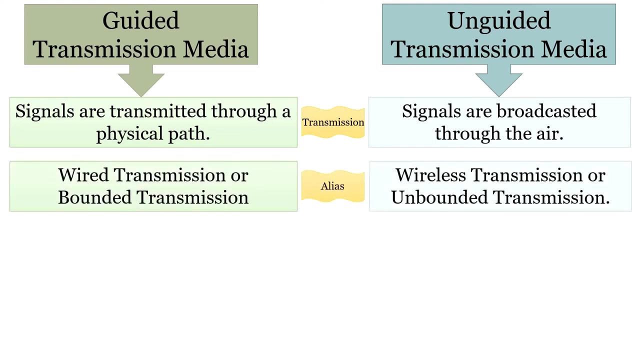 Knowing about guided and unguided transmission media in detail, Now let us discuss differences between them. The guided transmission media uses a physical path or conductor to transmit signals, Whereas the unguided media broadcast signal through the air. The guided transmission media is also referred as wireless transmission. 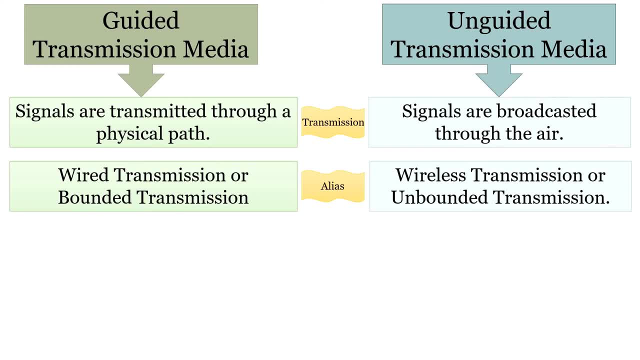 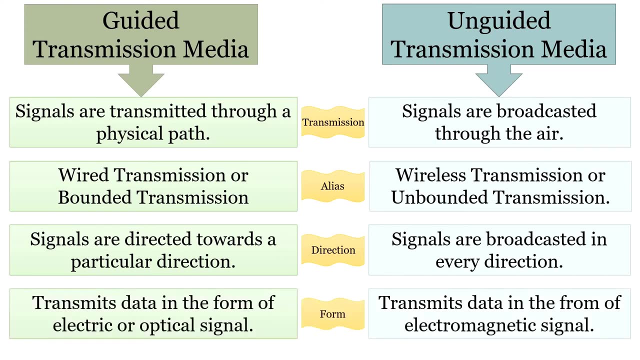 Or bounded transmission. However, the unguided transmission media is referred as wireless transmission Or unbounded transmission. The guided media provides direction to the signal, Whereas the unguided media does not provide any direction to the signals. In guided media, data is transmitted in form of electric or optical signals. 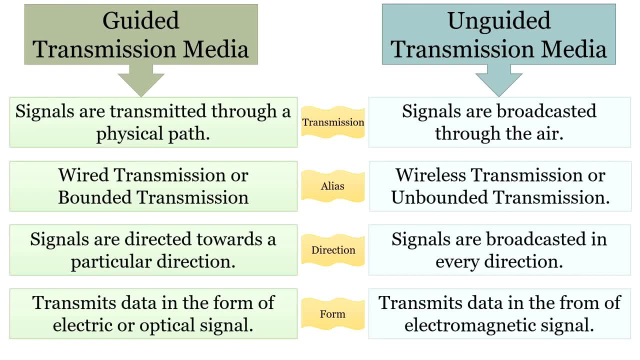 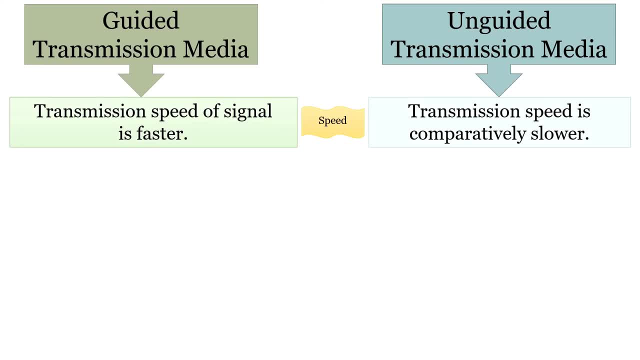 Whereas in unguided transmission media, data is transmitted in form of electromagnetic wave. Data transmission is faster in guided media, Whereas in unguided media it is comparatively slower. Guided transmission media is secure, Whereas unguided transmission media is comparatively less secure. The guided media is less harmful for human health.